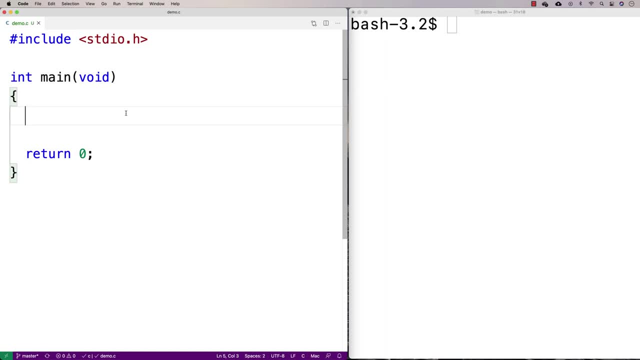 In this video we're going to go over how to count the number of occurrences of a value in an array, And it could be different kinds of arrays, but we're going to go with int arrays. So we're going to say int myArray is equal to, and we'll make our array with some values in it. so we'll say like 4. 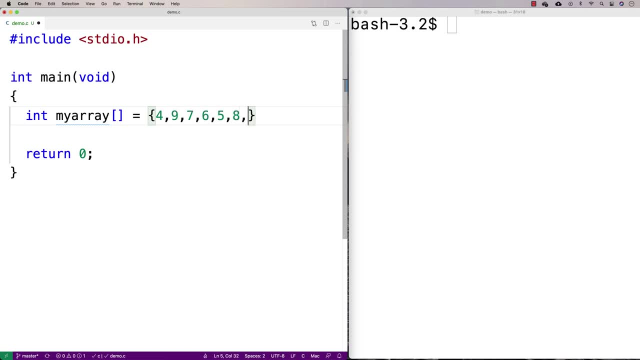 4, 9, 7, 6, 5, 8, 3, 2, 1.. And we've got what 1, 2, 3, 4, 5, 6, 7, 8, 9 values in here We'll add one more. 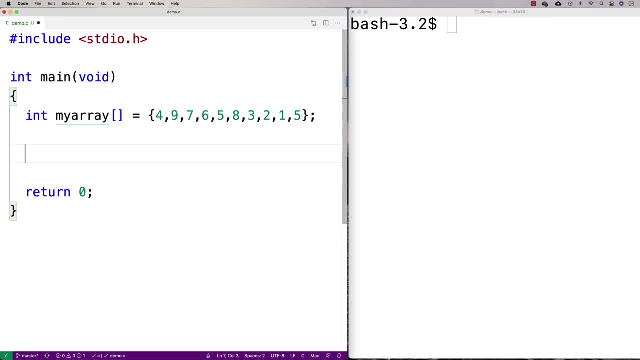 we'll add like another 5 there. So we've got 10 values in there now, And what we're going to do is we're just going to have a count variable that's going to keep track of the count. So we're going to say, int, count is equal to zero, And what we're going to do is we're going to count a. 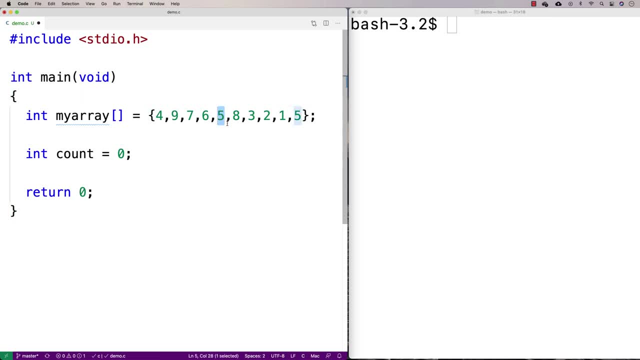 particular value that we want to find in this array, And every time we encounter it, we're going to increase the count by one, And what we'll do is we'll loop through the array elements. So we're going to start off with the first element and check all the way up to the last element. 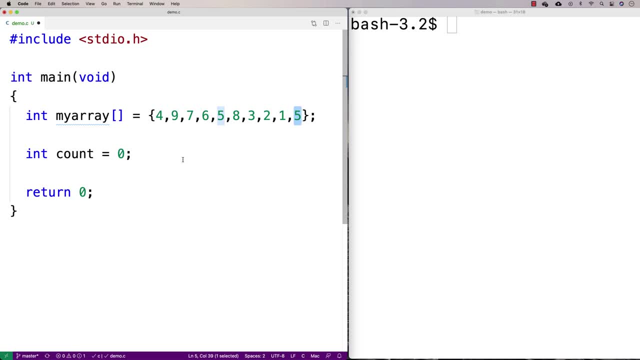 And we're going to just make sure that we check for the value that we want to find And we can make a variable with that. We can say like int, and we'll say: to find is equal to, maybe we'll say 5. And we'll make. 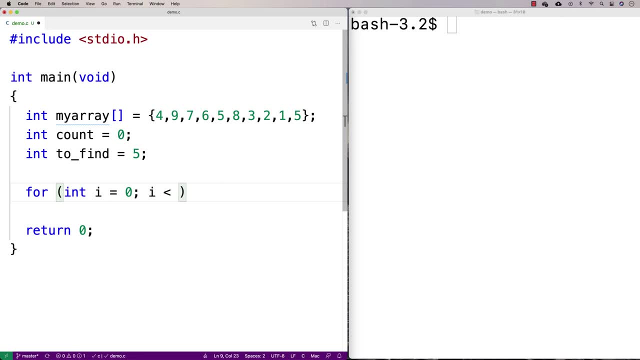 our loop now. So we'll say int i is equal to 0.. i is less than I've got 10 things in my array: 1, 2, 3, 4, 5, 6, 7, 8, 9, 10.. So I'll say less than 10, i plus, plus. And then I'm going to say if my array at i 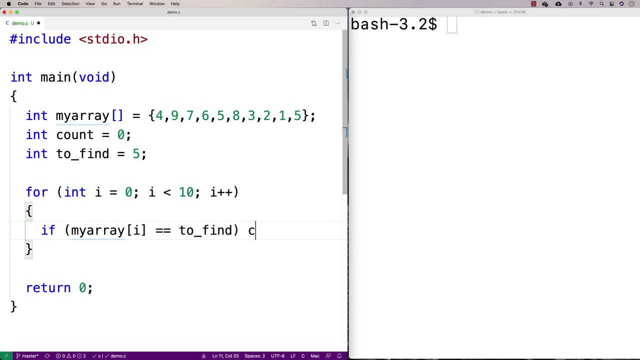 is equal to the thing I'm trying to find, then increment the count And then I should be able to print out the number of 5.. So I'll say like number of 5s found And I'll say percent d And then I'll output the count. 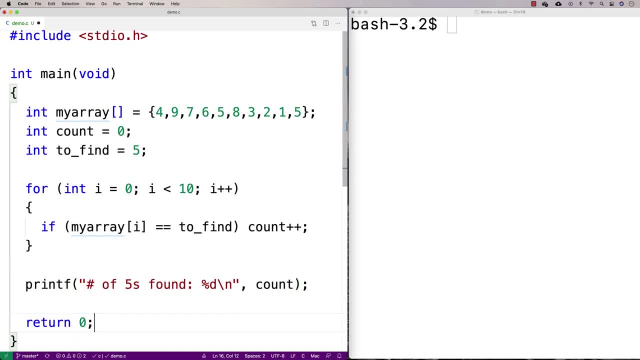 And we'll just say number of 5s found. Okay, So let's try to run this and see what happens. And I get: number of 5s found is 2.. If I were to change the to find number to say 6,, there's only one 6 in there. 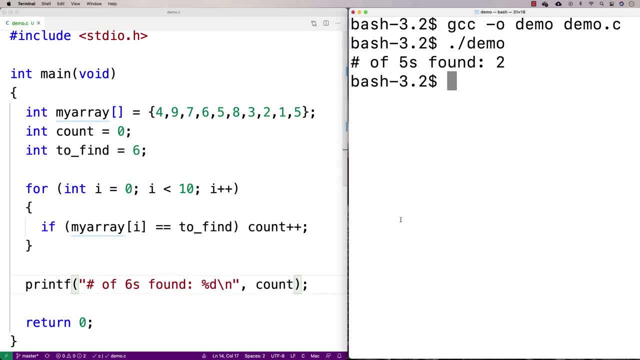 And it should then be that the number of 6s found is 1.. So I'll run this again. Number of 6s found is 1.. If I were to add, maybe let's change the 6 to: we'll just add a couple more 6s in there. We'll. 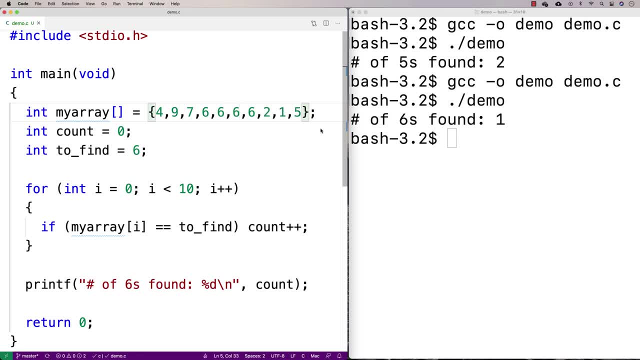 add like a 6 here, a 6 here, a 6 here, And now we've got 4 6s in there, So we'll give it a shot. now We got 4 6s, So our algorithm appears to be working And all we're doing is we're just checking. 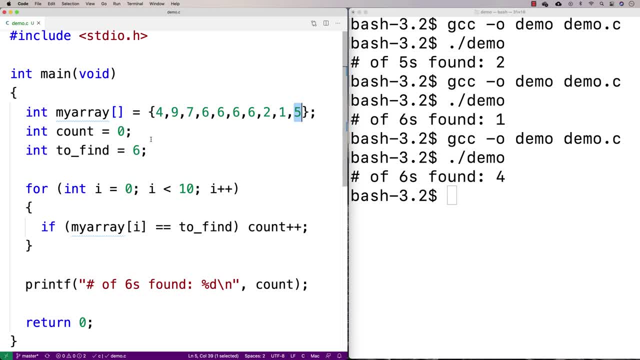 up until Index 9, because arrays start with Index 0. And we just check every value in the array to see if it's equal to the value that we're trying to find, And if it is equal to it, we increment count, having started off count at 0. So it's a pretty simple algorithm, But it is an algorithm. 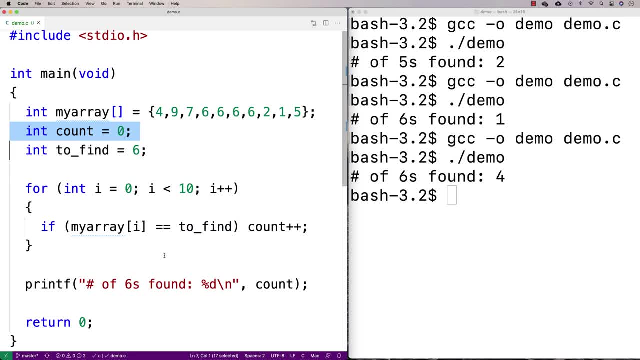 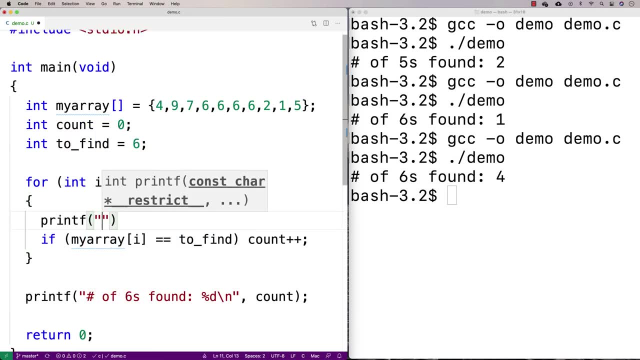 And if you're ever stuck on how to interpret how your code is working, you can always just throw in printf's to figure things out, So like if you were to- if you were to, you know, throw in printf's here you could check to see what array element you're. 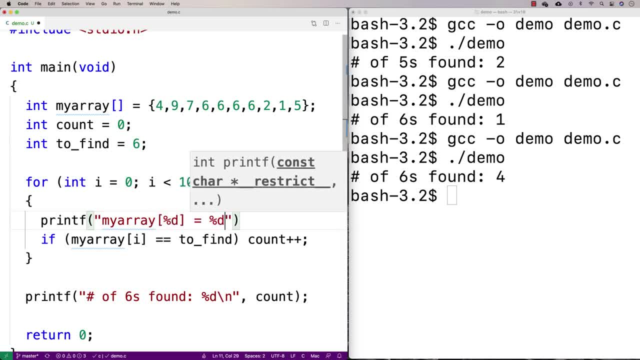 checking. So we could say: my array element is going to be like 0 and if I were to like, open it up, percent d is equal to percent d and what we could do is we could output i and we could output my array at i. so that way we know, you know, what array element are we checking now and what is its value. 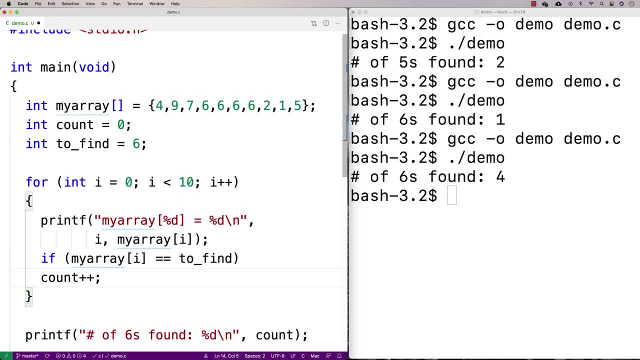 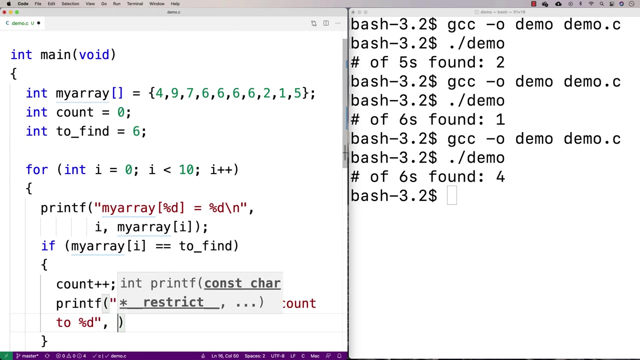 we could also throw like a printf in here to say that you know we found a value. so we could say like printf, we could say: you know, found percent d, um incremented count two, and we'll say percent d and then i'm going to say here: um. 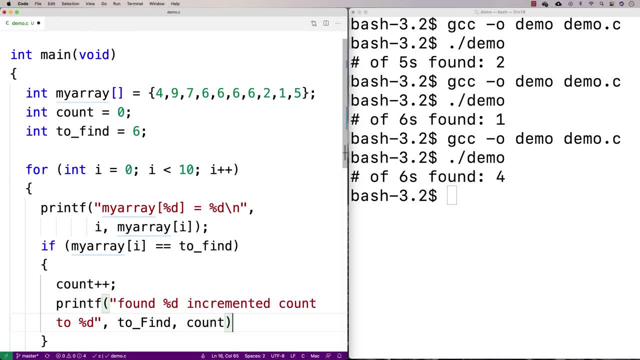 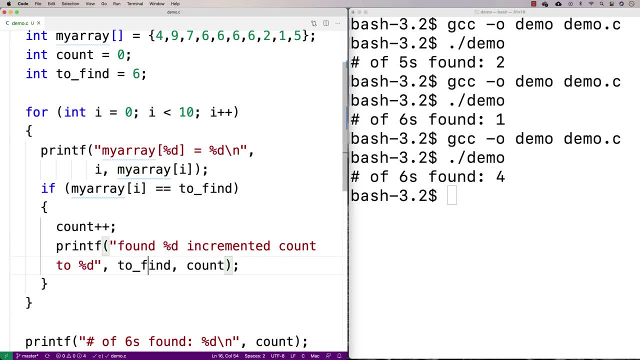 to find and we'll say we'll put the count. so here i'm saying like printf: found percent d and i'm going to put to find and we're going to say incremented count two percent d and we're going to, we're going to output the new value of count. 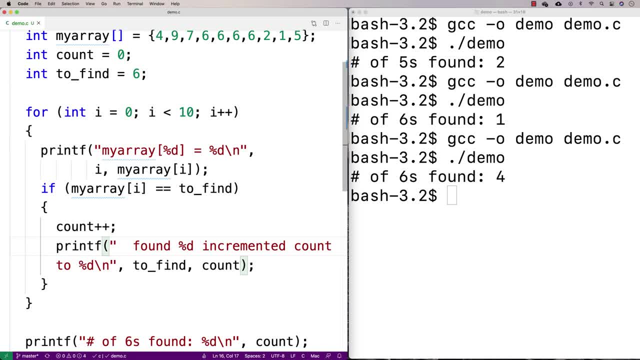 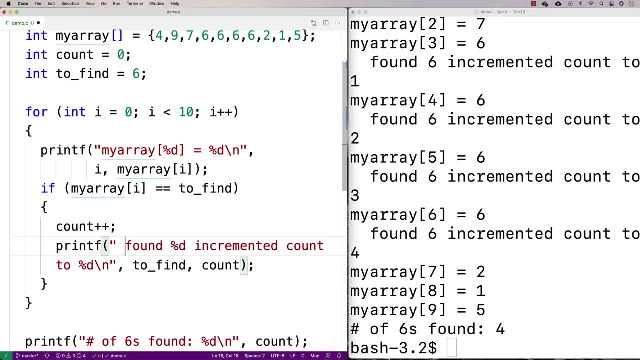 maybe let's put a little tab here too, just so we can kind of make a special note of it here. so if i run this here now, right, what you can see is: you can see, and maybe actually i'll take that back, just that way it gets on one line again. it kind of it kind of squished things a bit in terms. 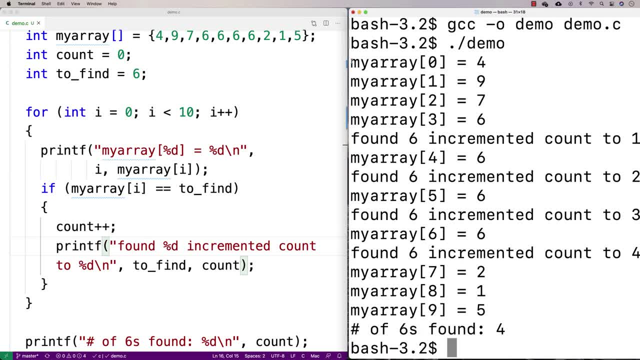 of the output. so we'll just do it again here, okay, so you can see here, um, you know, we check my array zero for four. we check my array one. it's nine, seven, six, okay. but now when we find a six, that's what we were looking for. so 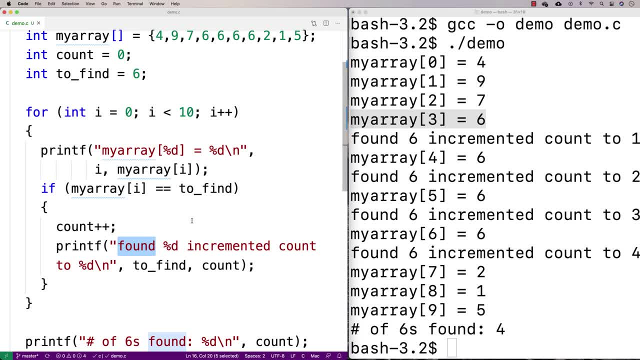 we output here: found six, increment account to one. and then here, you know, we find another six: found six, increment account to two, increment account to three, increment account to four. and you can see what's happening in our code with these print f's, because they're letting us know, you know that. 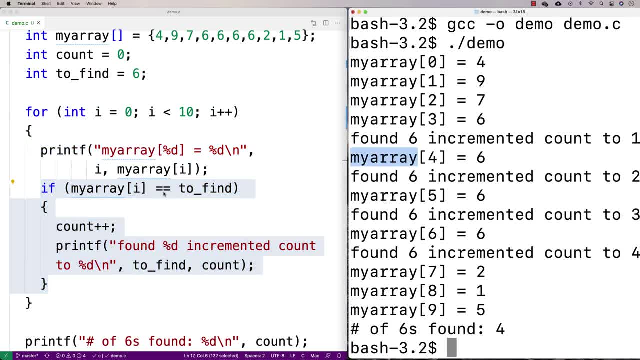 this: if statement is running because we are encountering a six and you can tell that it is a six at that in the array at that position, because we're also outputting that information, we're outputting the array index and the value at that index for this iteration of the loop here. 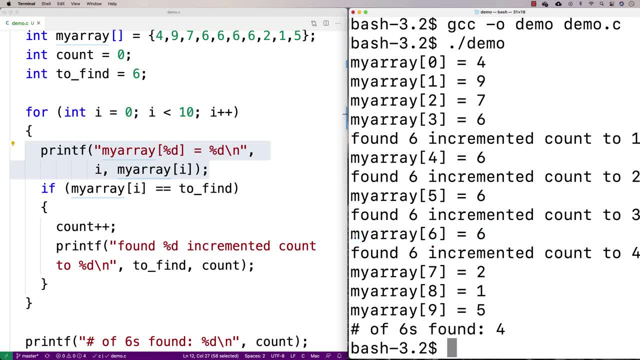 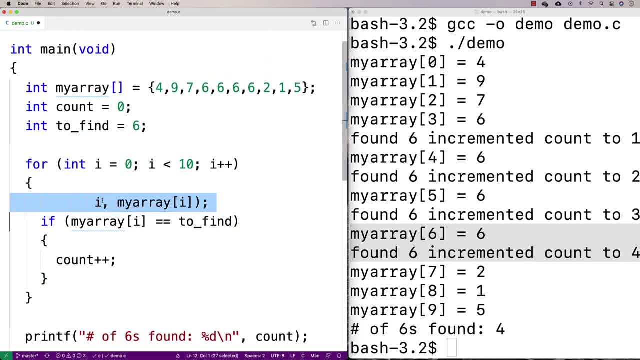 so we're able to see that like, oh, we found a six and it makes sense because there is a six here. um, and so whenever you're you're having trouble understanding how your code's working, throwing in printfs is always a good idea, to just to just. 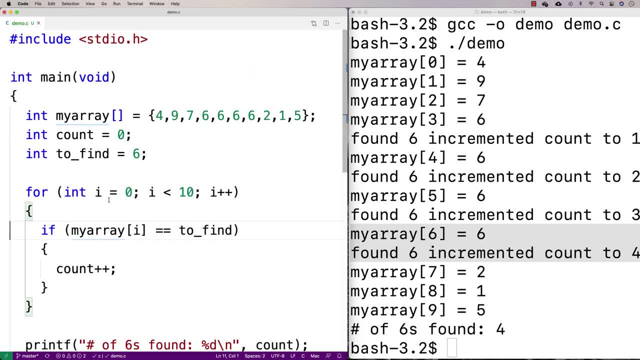 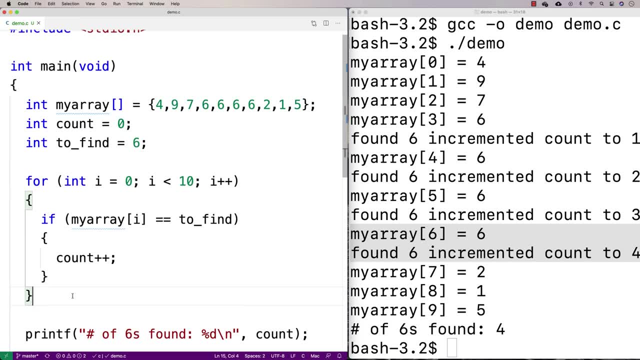 understand. you know how your code's actually functioning. now, one thing we might want to do with this here is put it into a function, so that way we can call it again and again whenever we need it, as opposed to, you know, writing with the logic once and then we'd have to repeat this in. 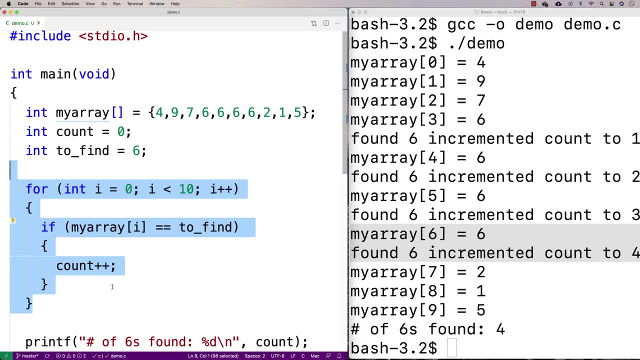 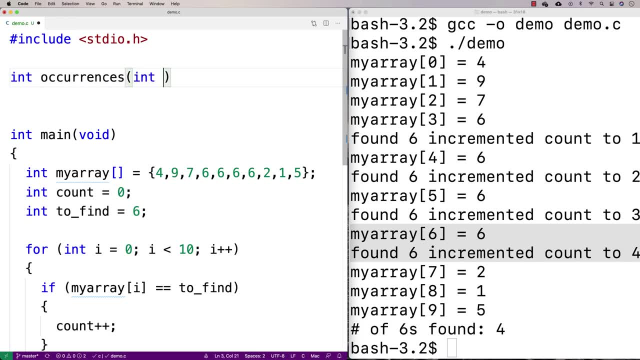 our main function wherever we need it. if we put it into a function, we can call it whenever we need it. so what i'll do is i'll make a function called occurrence is so we'll say int occurrences, and it's got to accept a few things. it's got to accept the. 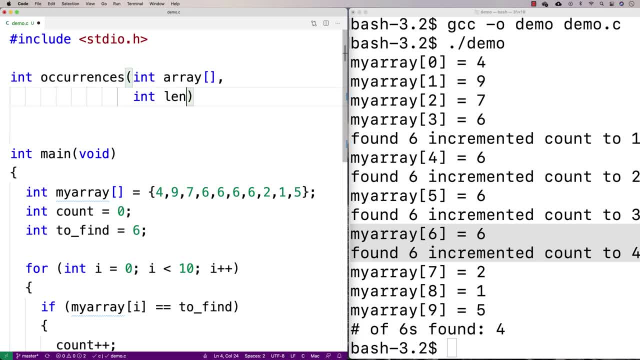 array as a parameter it has to accept the length and it's also going to need the value that it should be finding the number of occurrences of. so it's going to need those parameters and we'll actually just kind of copy and paste a lot of logic here, because we've already kind of worked. 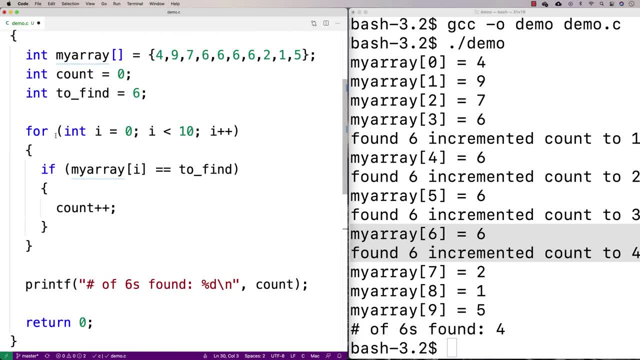 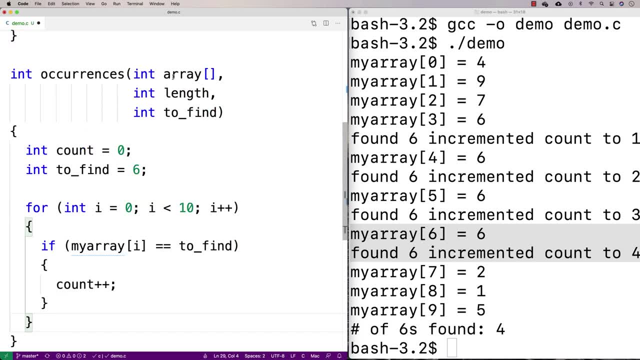 it out. we might as well- just you know- use it again here. so i'm just going to copy and paste this in, just. for the most part it'll work. the only difference is i called it array here, so i'm going to change it to array there. 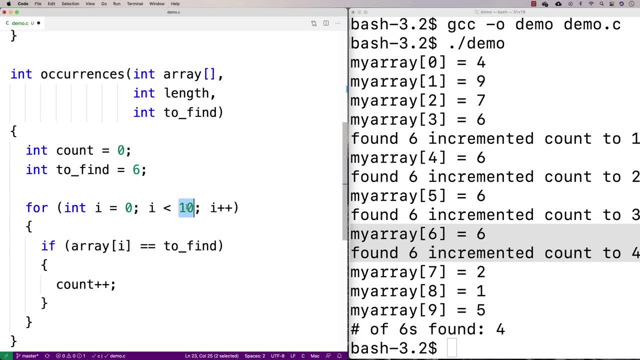 and the length is now not set to 10. the length is going to be a parameter that we pass to the uh. it's going to be a parameter that the function has, so we're going to pass it as an argument. so we'll say here: uh, i is less than length, so that way it'll work for any length and i'll. 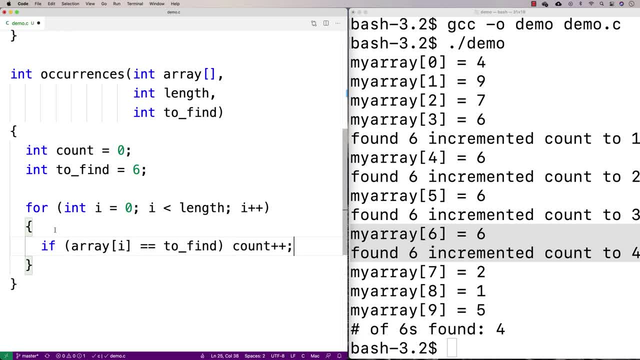 just throw this up on one line again. and you know what? i could even just put this on one line too, because really the for body only has one statement, so i might as well just put that on one line too. squiggly brackets just to make the function concise And to find is no longer being accepted. 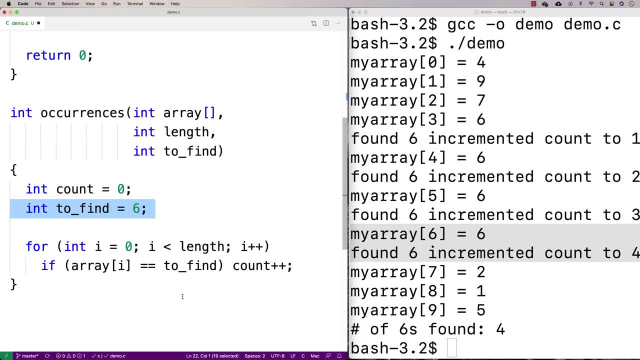 as a parameter. It's, or, sorry to find, is no longer a hard coded, I should say to six. It's now being accepted as a parameter. right, So to find I should. I should actually get rid of that. 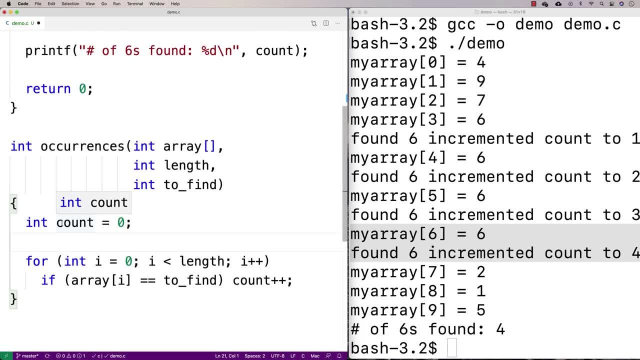 there too, And and now it's. it's basically a simple function where we just start off with count being zero, We loop over the loop length, We loop over the array length and then we check to see if the array at the position is equal to what we're trying to find. So I've got one array. 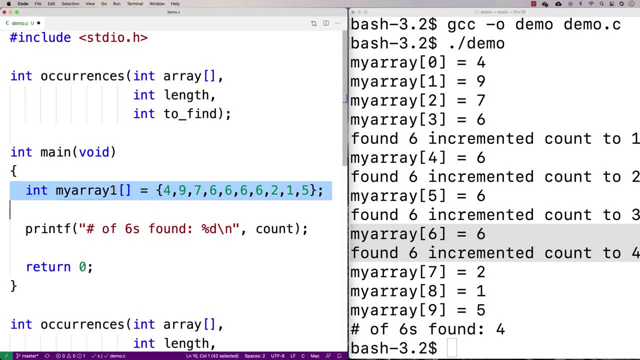 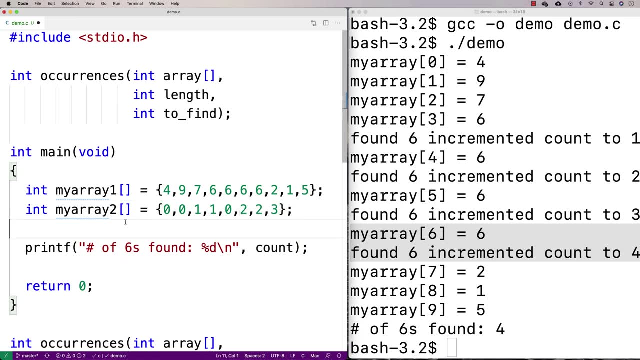 there. I'll make another array here, just so we can test both of them. So I'll say like int, my array two, and I'll make this other array have some different values in it. So maybe we'll have like zero, zero one, one, zero two, two, three. And what we'll do is we'll we'll check the. 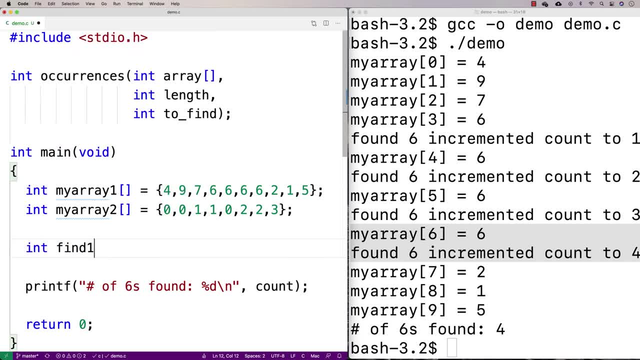 occurrences of a couple of things. We'll say like int find one and we'll try to find like fives in the first array And I'll add it. I'll add in another five just to make it more interesting, or add in two more fives just to make it more interesting. 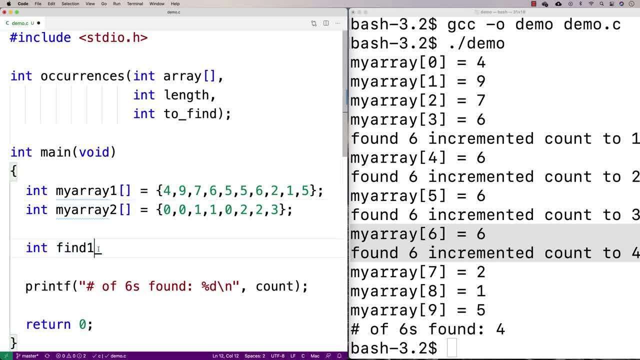 So we'll try to find fives in the first array. So we'll say find, find r. one five is equal to, and we'll say occurrences, and we have to pass it my array one, And we're going to have to pass it the length of the array, which should still be. we had what was. 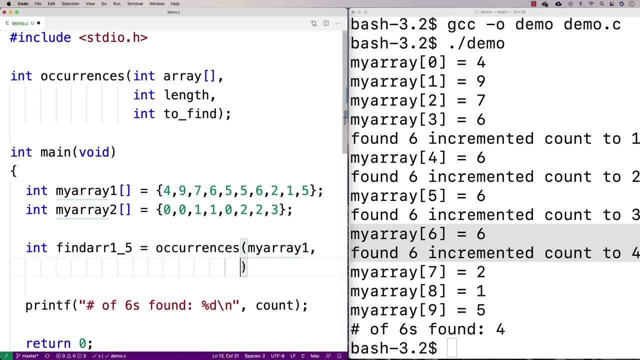 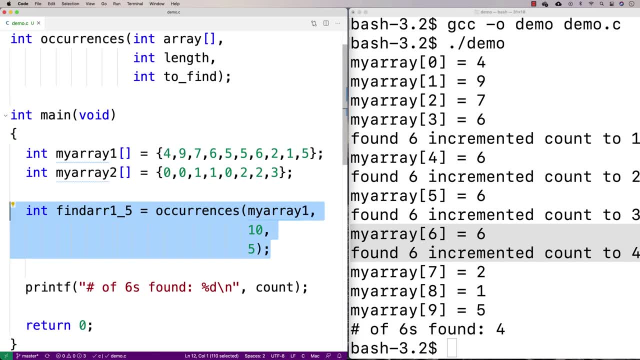 one, two, three, four, five, six, seven, eight, nine, 10.. So the length of the array is 10.. And then we'll do the same thing for the next array: We'll try to find the number of zeros in this. 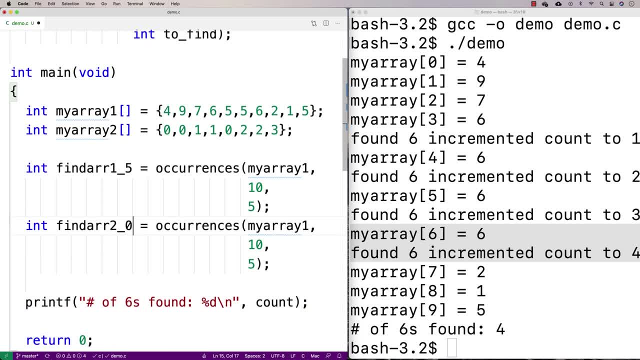 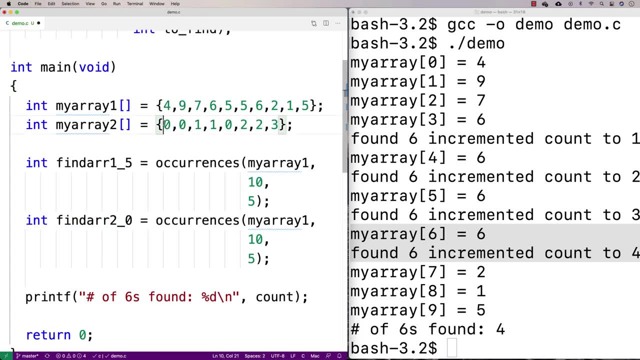 array. So in array two we're going to try to find the number of zeros And I just kind of- this is just my like little convention here- just to keep track of like what I'm, what the value is that I'm finding, And I'll just say here how many, what's the length. here We got one, two. 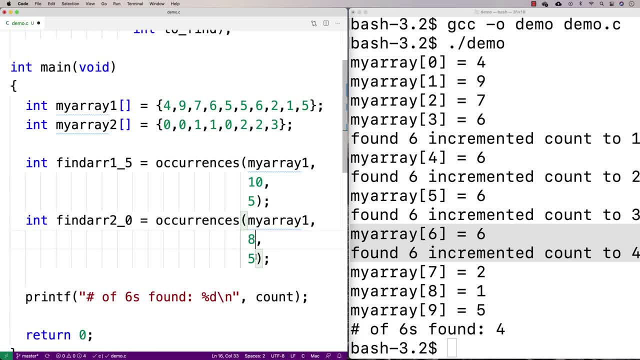 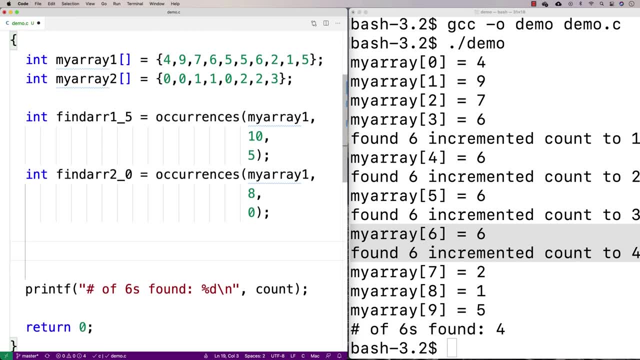 three, four, five, six, seven, eight, So eight things in the array and we're going to try to find zero. Okay, So then here I can print out. we'll say print f, we'll say number of fives found in array. one in my array. 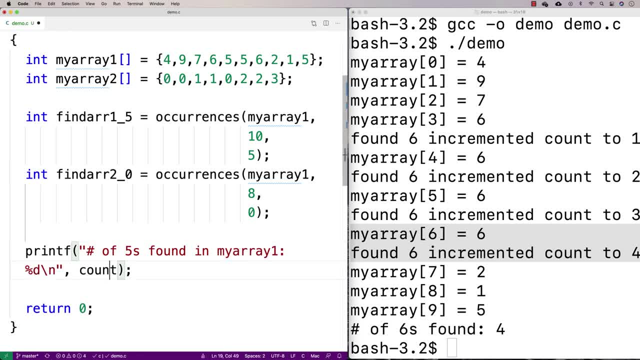 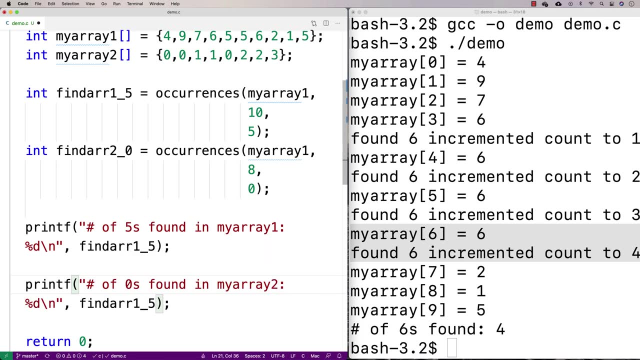 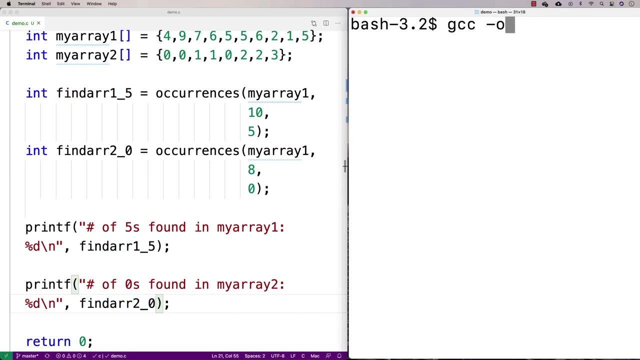 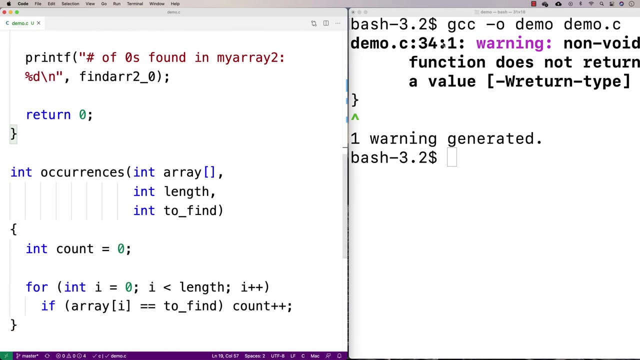 one is going to be find our one, five, And then we'll we'll print out the number of zeros found in array two. So print out number of zeros found in my array two And that one we called find array zero. Okay, So we'll clear this. give this a try. Warning: Oh, I didn't return. I just saw that. 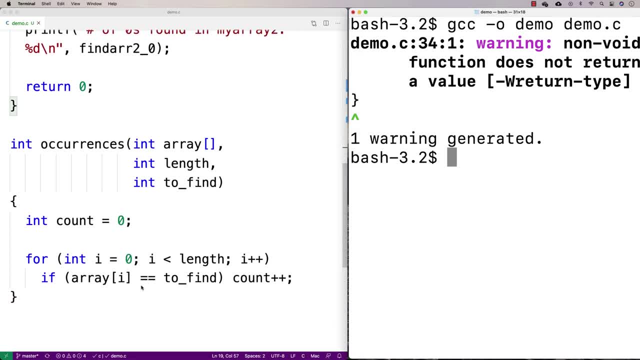 error there. It says: warning: non void function does not return a value, right? I forgot something important here. This function has to return the count. That's pretty important that the function that's supposed to count the occurrences returns the actual count, And I forgot that, So I've added. 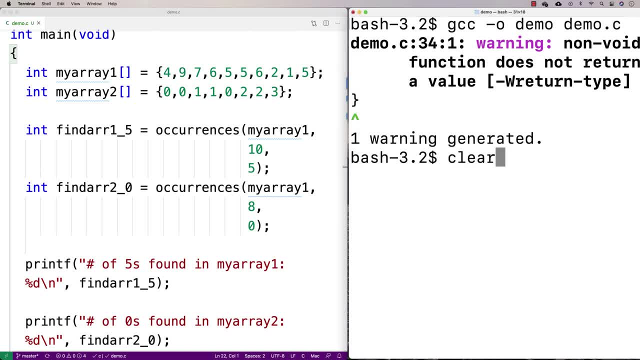 that in there, there, there, now, Okay, So that should fix that. Let's give this a shot And we get that. the number of fives found in my array one is three And the number of zeros found in my array two is zero. That's because I passed in my array one instead of two, So it says: 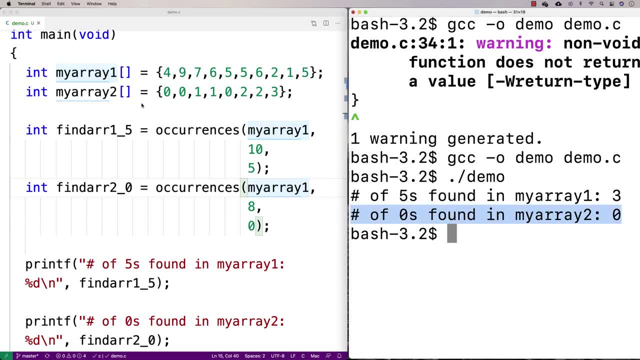 I was kind of surprised by this value because it says number of zeros found in my array two is zero. But if you look here, I actually didn't pass in my array two to the to the second function call. I passed in my array one. If I do pass in two it should find zero. We'll give this a try And now. 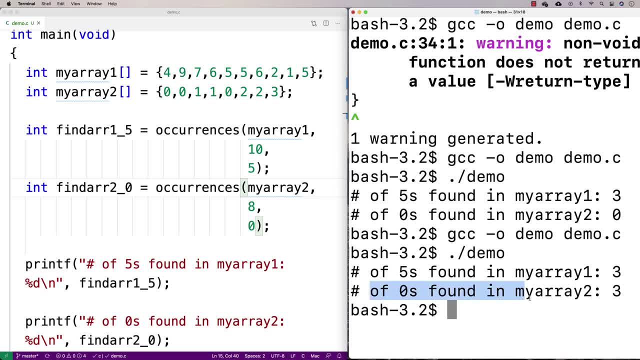 yeah, it's out, So it's. it found the three fives in the first one and the three zeros in the second one. We could mess around with the values, Like I could put in a couple more fives in the first one and I'll put in a couple more. I'll put in like one. 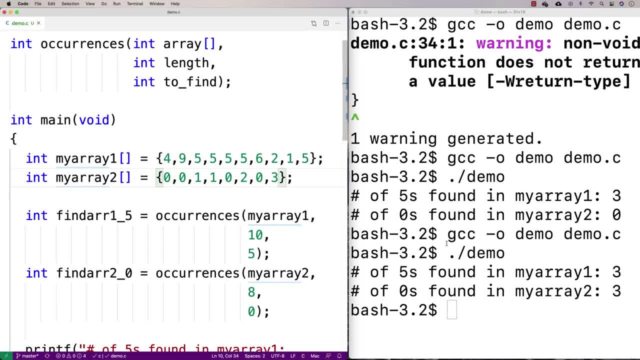 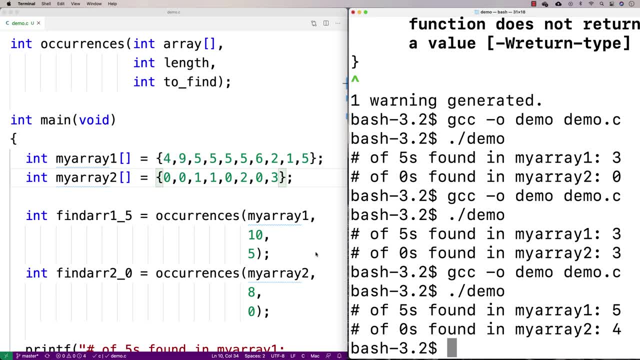 more zero in the second one, And you know, I can run this and we can expect to get the same correct result back. So we've got five, fives, now four zeros back, which makes sense. And so now what we've done is we put in this this function that we could then 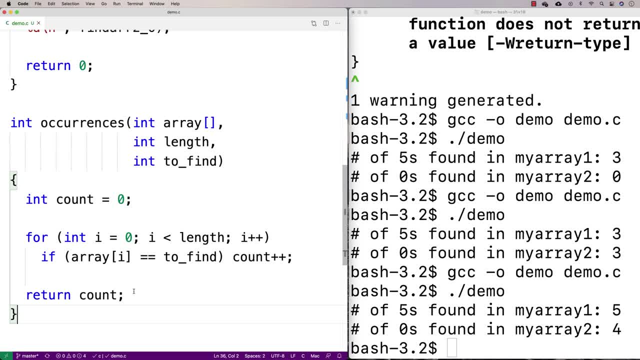 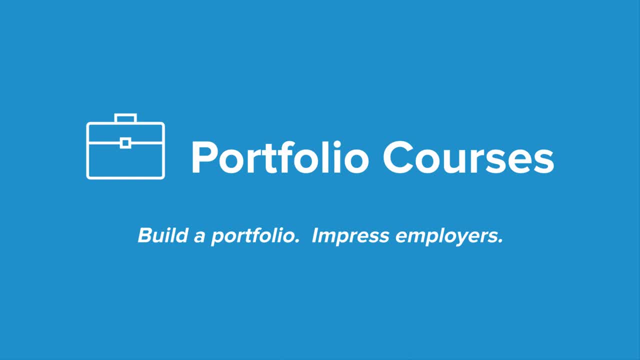 use again and again wherever we need it, And so if we're going to try to solve this problem, this would be a good way to do. it is to put in a function so we can call it wherever we need it. Check out portfolio coursescom, where we'll help you build a portfolio that will impress.